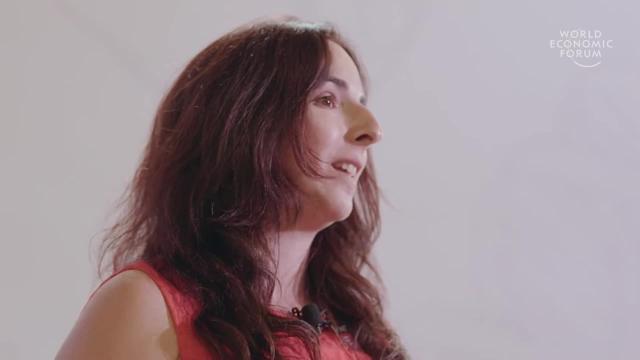 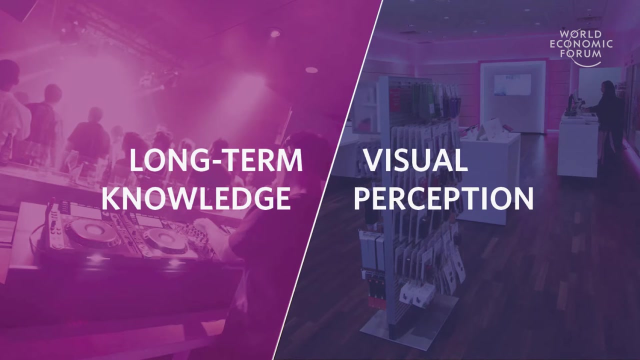 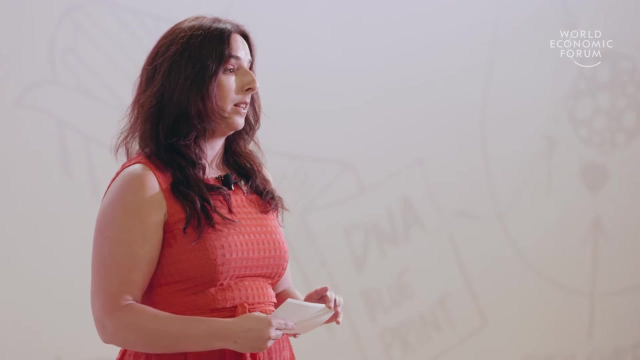 But most of the time we are successful in our predictions And therefore our visual experience comes from not just a veridical analysis of light falling on our eyes, but rather an intermingle of our lifetime of experience and our perceptual input that gives rise to. 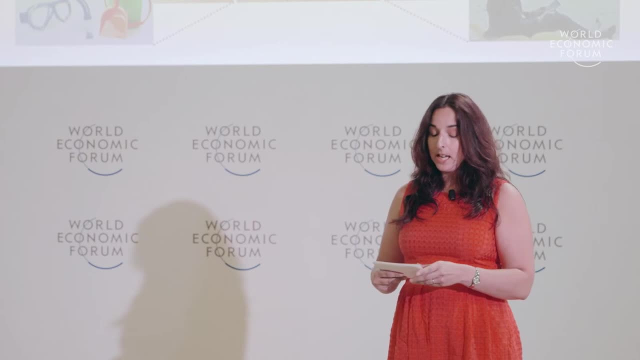 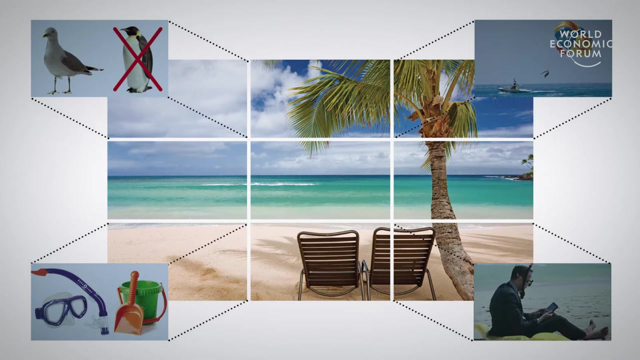 our visual experience. So what does it mean to see, What does it mean to understand our visual world? It means going well beyond just looking at a scene. For example, because this is a beach scene, we have certain expectations and stereotypical associations of objects. 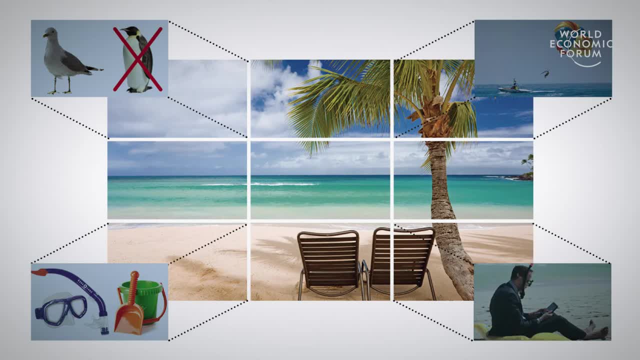 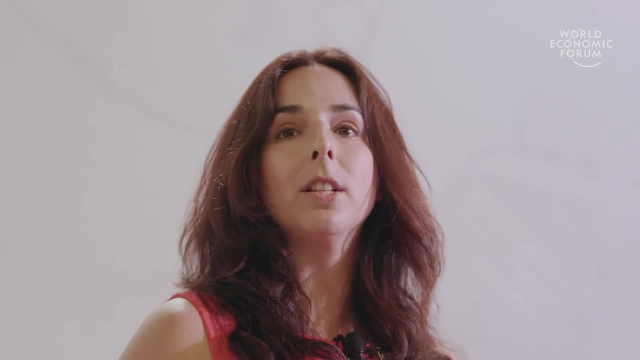 that we expect to see and certain actions and behaviors, And therefore to see is not trivial. Computers are still bad at this problem. Although there has been amazing progress over the last few years, computers would still have a hard time telling you why a 40-foot 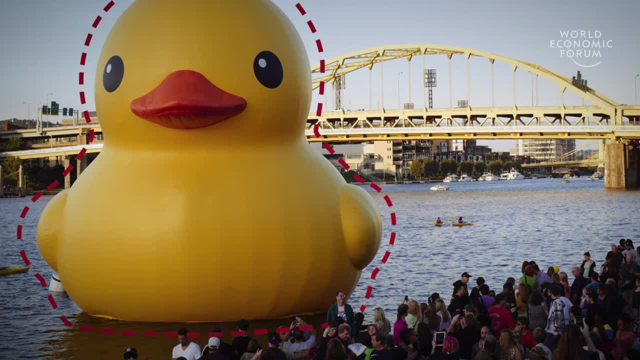 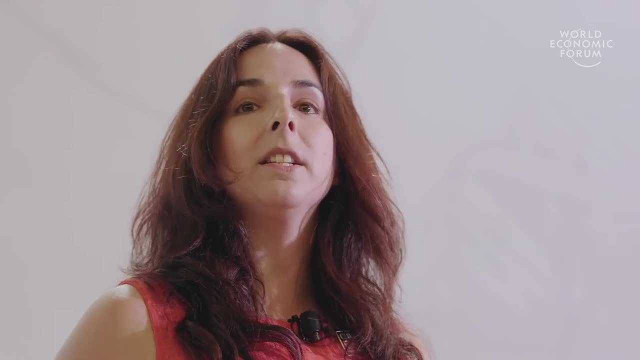 rubber duck in a river is unusual. I want to understand how we are so good at this problem- And by we I mean our brains, of course- And the place to look for answers is a network of brain regions that process the visual environment. 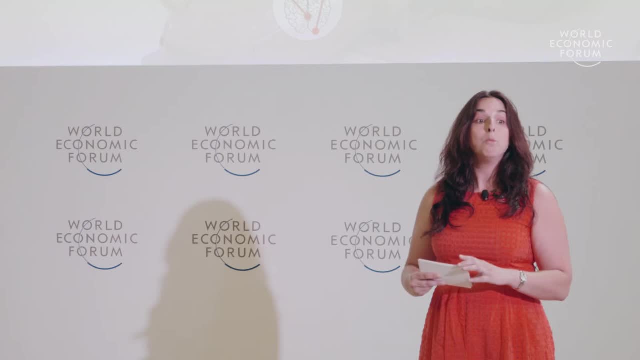 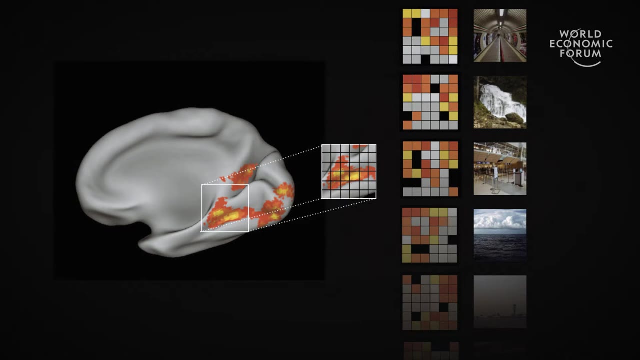 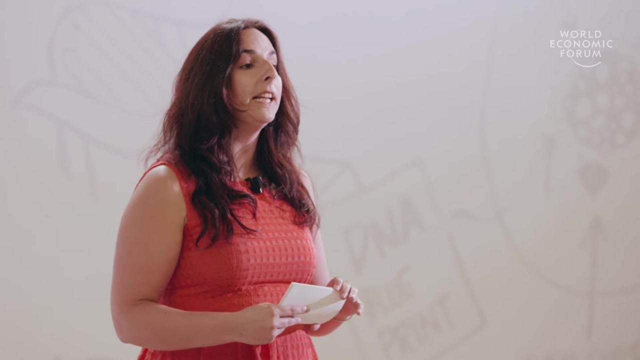 These areas process stimuli such as scenes like a beach more than other stimuli, such as faces and nonsense images, And, moreover, these areas don't process scenes all equally. The differences in brain response between scene stimuli can reveal meaningful clues about how the brain represents information about a scene. 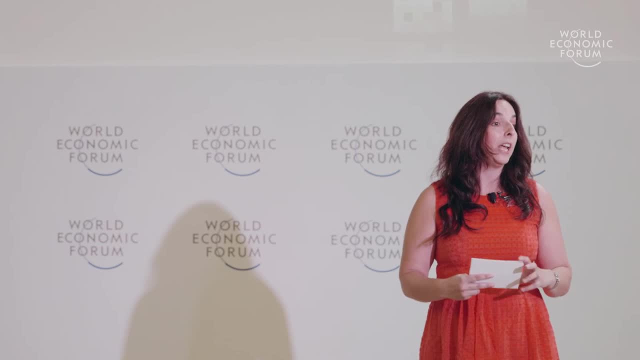 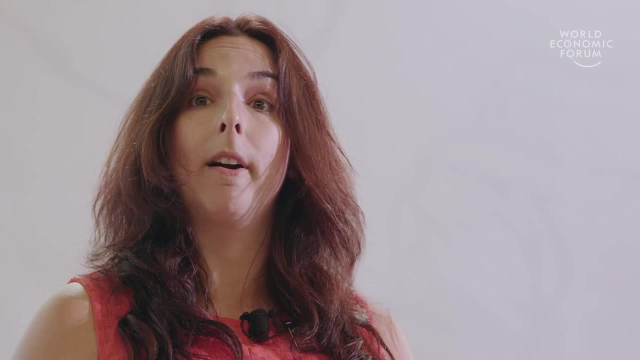 And it can help reveal the code the brain uses in order to understand our visual world. For example, a key question is: how does the brain break apart a scene? What are those visual nuggets that help us predict what else is going on in the scene, Just like a sentence? 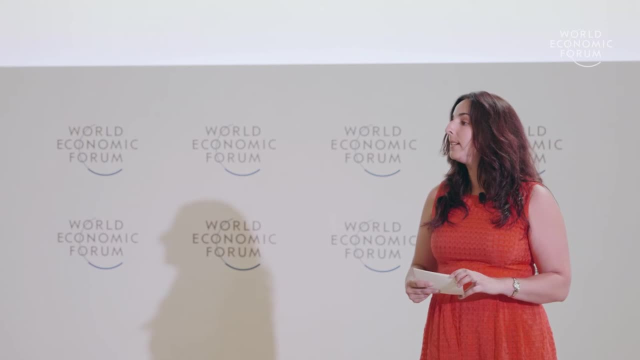 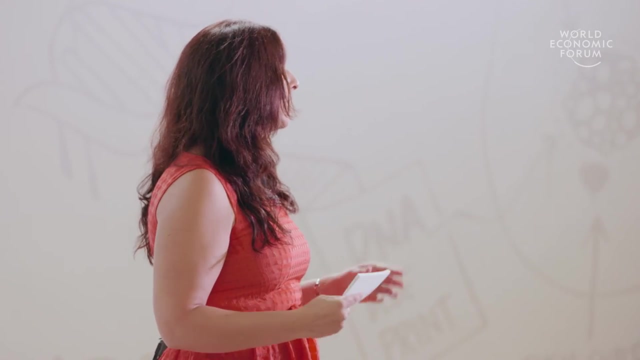 can be broken down into words. how can a scene be broken down into meaningful units? If we could answer this question, we might have a better idea of how the brain represents scenes. We have terrible self-reflection about how to explain our brain processing, So therefore. 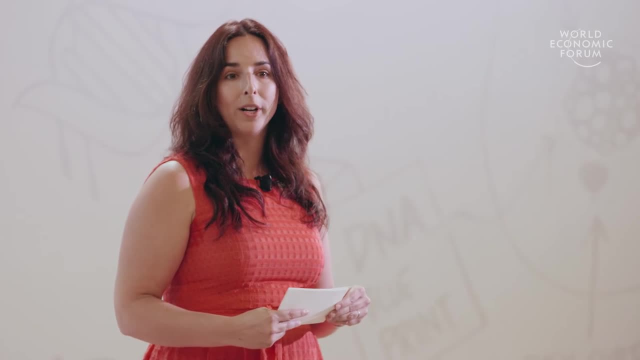 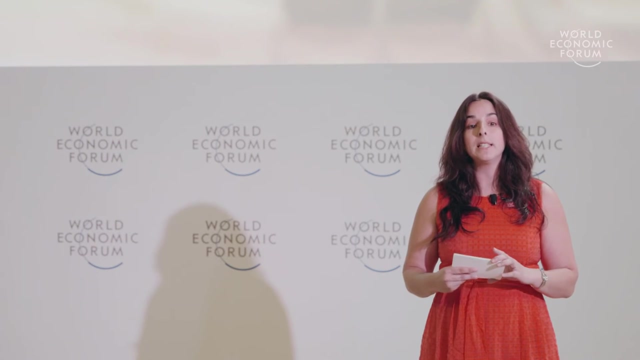 we can't just sit in a chair and decide what are the most important aspects of a scene. How does the brain understand what are the critical parts of a scene? By having a lifetime of experience analyzing scenes, As I like to say, the brain is the biggest big data.